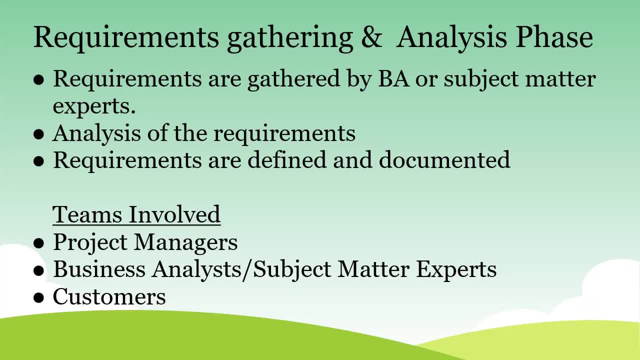 Later these requirements are defined and documented in the proper documents. If it is the requirements from the customer, that is, if it is a business requirement, then you have to come up with business requirement document. Or if it is a system requirement, then you have to develop system requirement specification document for this. 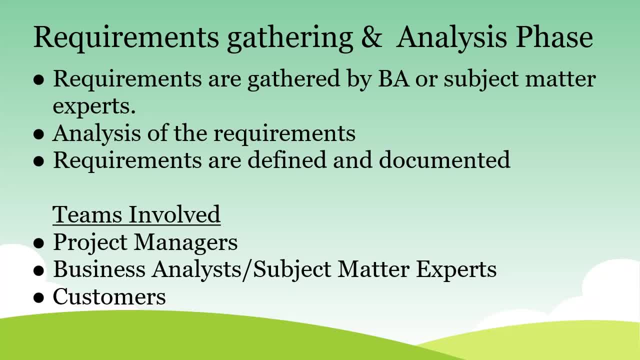 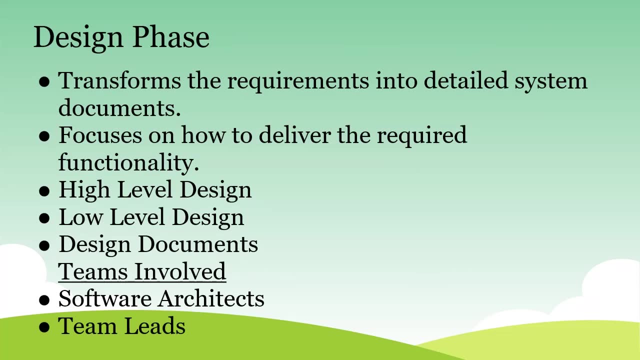 And there are different team members involved in this particular process, like project managers, business analysts or subject matter experts and the end customers. Now let's look into the second phase of SDLC, that is, Design phase. In Design phase, we are actually transforming the requirements into detailed system documents. 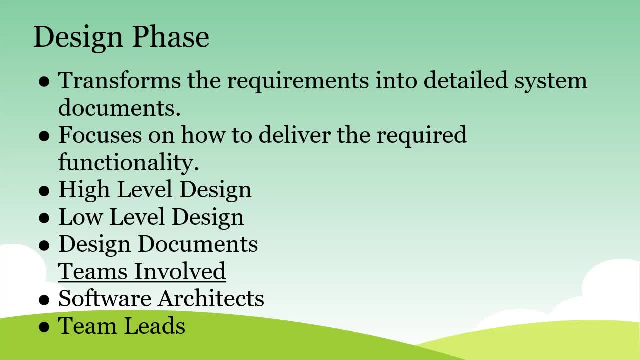 It is actually focusing on how to deliver the required functionality, And there are two types of design phases, that is, high-level design and a low-level design. In high-level design, we are coming up with high-level design document And in low-level design, we are actually preparing the low-level design documents. 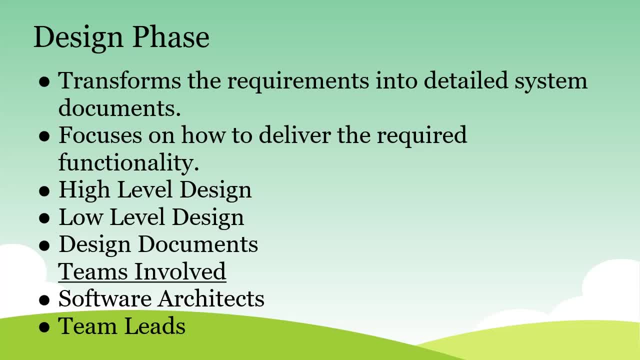 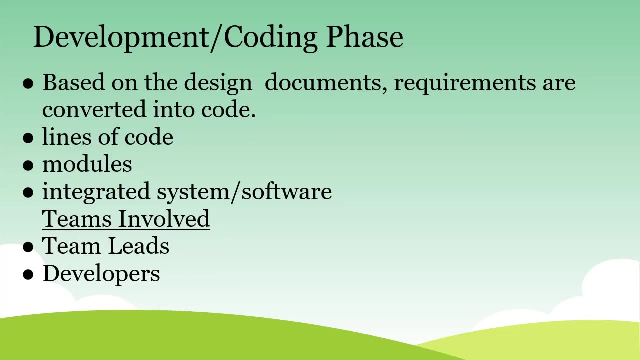 After the design phase we have to come up with the proper design documents. The teams involved in this particular phase are mostly software architects, team leads etc. The third phase in SDLC is Development or Coding phase. In this development or coding phase the real programming happens. 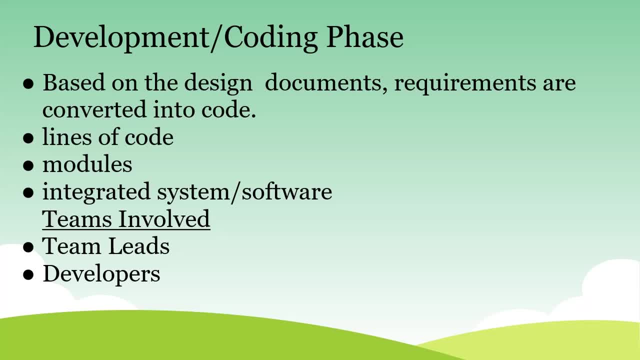 And, based on the design documents, the requirements are converted into lines of code And, for the ease of development, the software system might have subdivided into different modules and for each of the modules different lines of code are involved. Later these modules are integrated together to form the system. 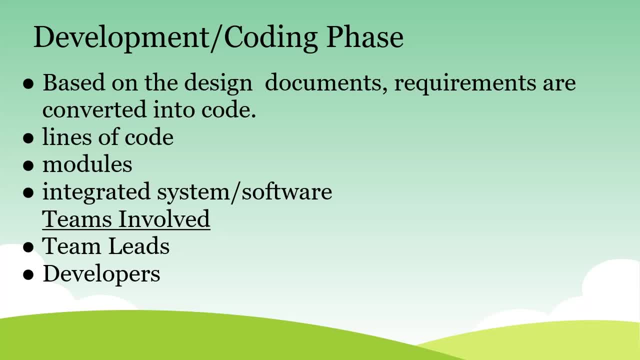 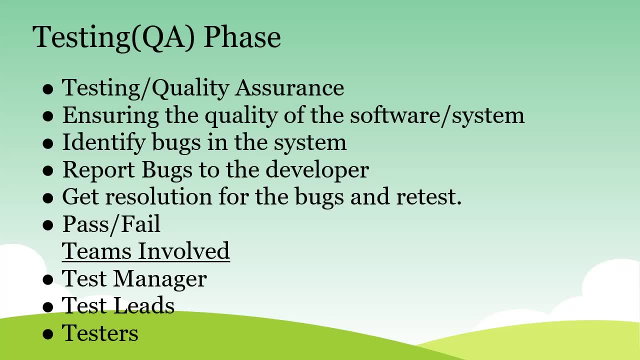 And the teams involved are mostly team leads and developers. The fourth phase of software development lifecycle is a testing or quality assurance phase. In this testing phase we are actually assuring or we are actually ensuring the quality of the end product, And it is the responsibility of the testers or the quality analysts to identify most of.